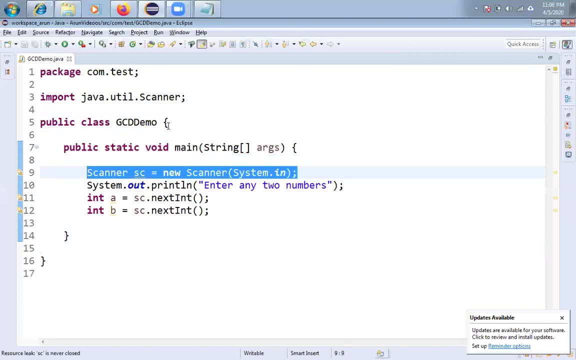 one main method and I created one object for scanner class and I am getting two values from the keyboard, say A and B. Now what I am doing is I am creating one method- name of the method It is called find GCD- and I am passing A comma, B value as well, See. mouse over this and create. 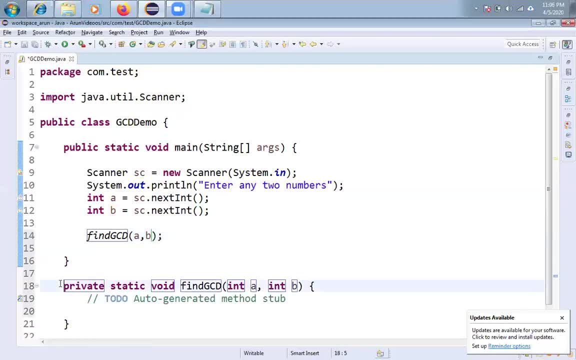 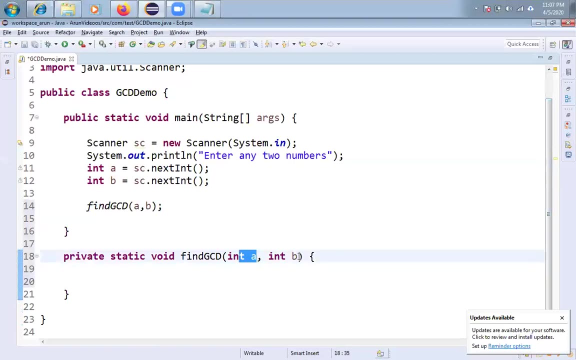 find GCD method. Automatically method will be created. So inside you can create, you can develop your logic or you can implement your logic. Okay, Whenever you are calling find GCD, then what will be happen? A value will be copied into here and B value copied. 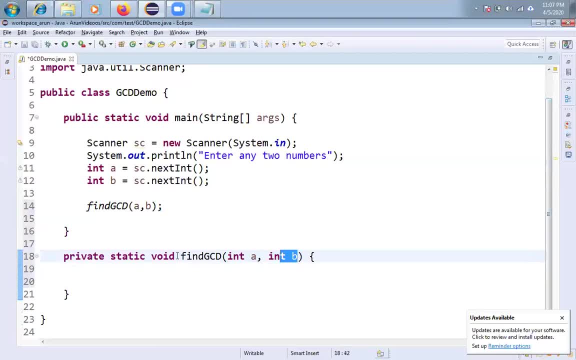 to this B. And one more thing: this find GCD- Why it means it is. it will not return anything, but I will return one major value. So what is the logic I'm going to use here? If you divide a value with the B, if you get remainder, 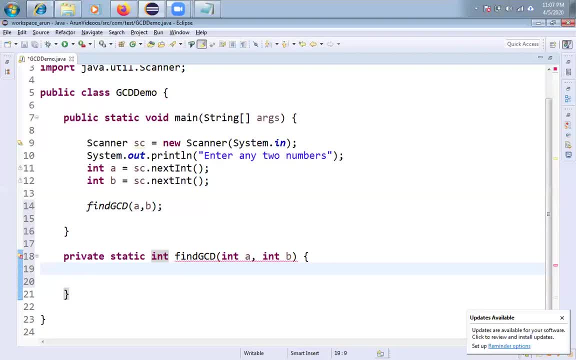 zero, definitely, I mean immediately I can say B is GCD. Okay, That is a logic. I'm going to check here: If a mod B equal to zero, so you can say you can return B value because B will become GCD. 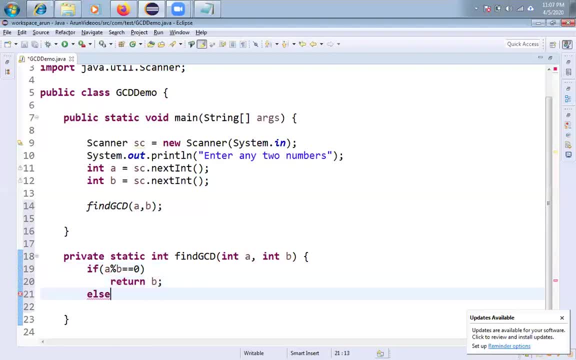 Yes, Yes, Yes. divide a and a with b. if you did not get, like remainder zero, then again i will call find gcd. in this case, what will be happened? a will become b and a will become b and b will become uh, i mean, remainder will become gcd. sorry, remainder will become b. so that's why a mod b i am taking and 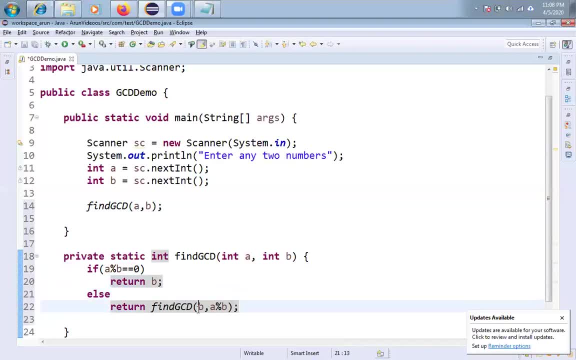 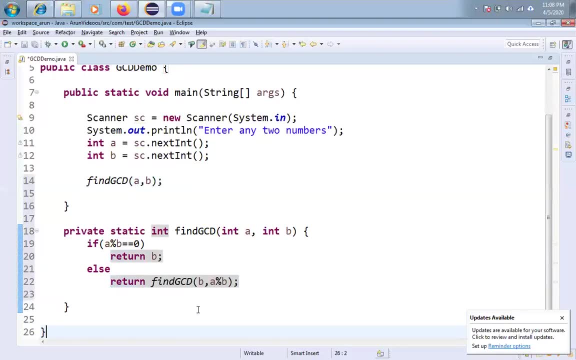 i am repeating once again in this case what will be happen: b will become a and b will become remainder. that's it, no confusions. and let me execute this one. before that, find gcd will give you one integer value. so catch that value- integer g equal to, and display that value here. so gcd equal to plus g.